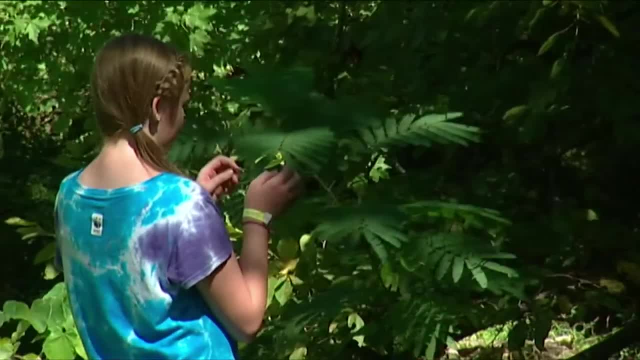 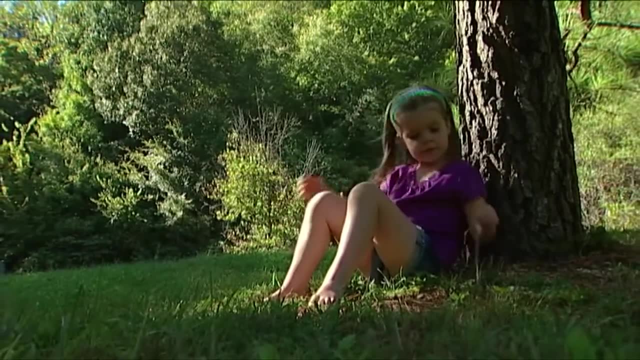 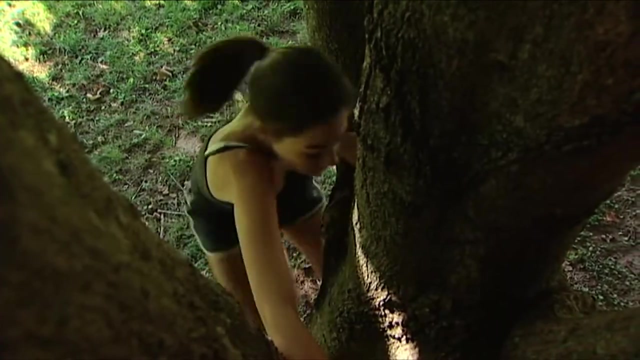 happen. mud pies can happen. Trees and shrubs can also feed your kids imagination. Having a secret or personal spot where a child can sit and daydream and enjoy the nature is a must. Enjoying some quiet time outside is important too, And don't be afraid to let them climb a tree. 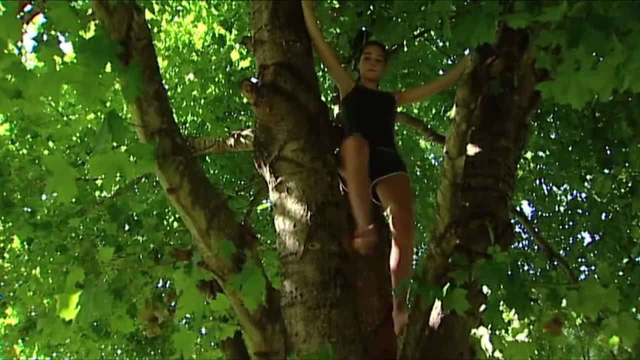 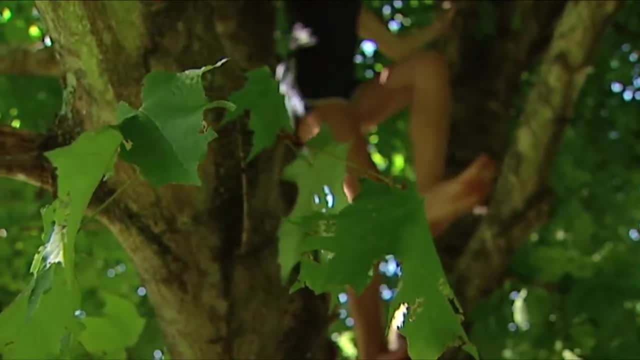 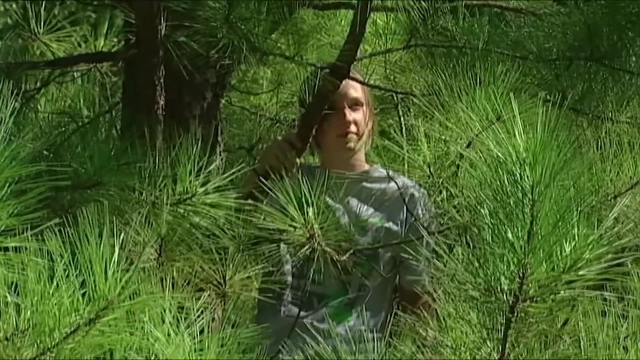 Just to be able to look out on the world and to feel the texture of the tree and see the bugs crawling on the tree and maybe see a bird light on the tree with them, Listen to the leaves, just become a part of it. That's an experience that is required for children. 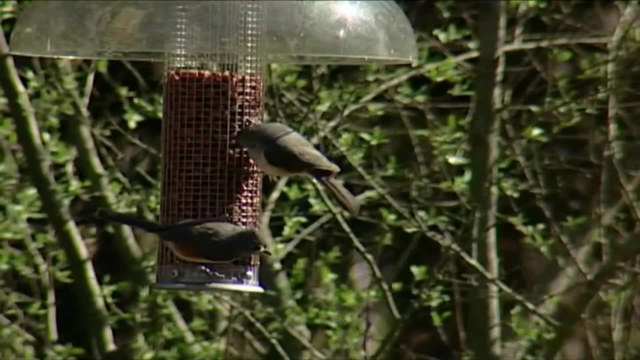 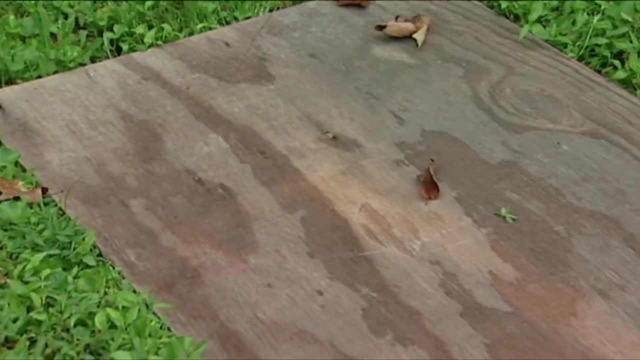 You can also make spaces for wildlife with bird feeders, houses or even a discovery board. Put a piece of wood, a board, down that's about two foot long, maybe about two foot wide, and leave that for a couple of days in a quiet place, And then, with 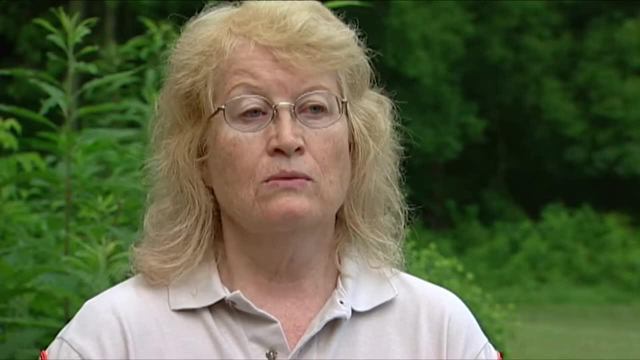 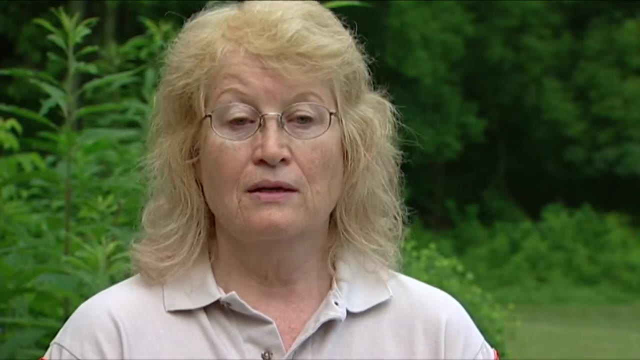 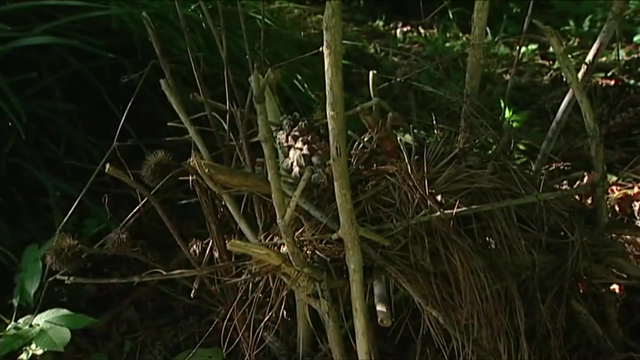 the child peep under it and see what neat things might have found a shelter there, And it could be bugs, it could be worms, slugs, it could even be a lizard. Another fun home kids can create is a hidden house for fairies. If you want to build a fairytale house for your kids, you can build a. 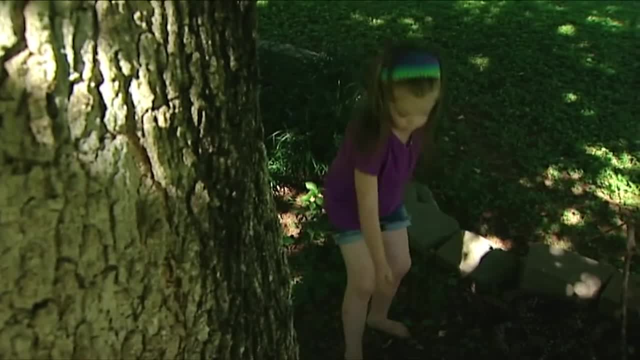 fairytale house for your kids. If you want to build a fairytale house for your kids, you can build a fairytale house for your kids. you can build a prairie house. You need to use the materials that are natural, the ones that are found right near that spot. You need to bring the 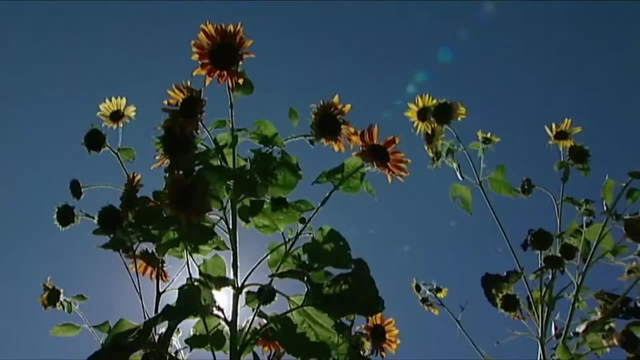 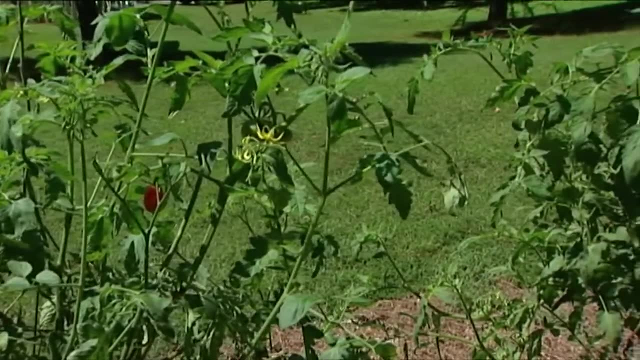 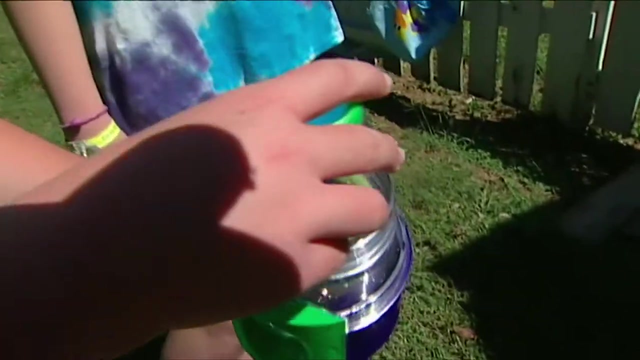 pebbles from nearby, the twigs, the leaves, the flowers. Planting flowers or even a small garden with your kids will help them understand the cycle of life and will attract all kinds of wildlife, especially bugs and worms. Magnifiers and bug cages are great tools for getting a closer look at 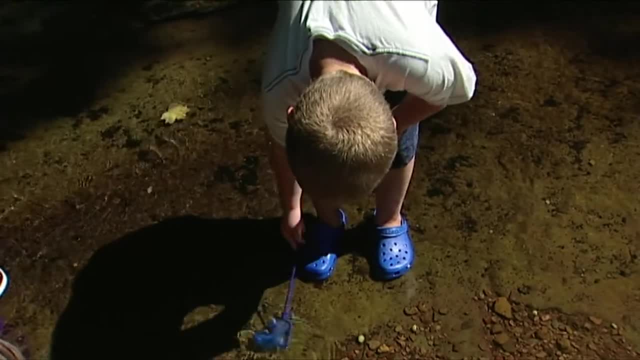 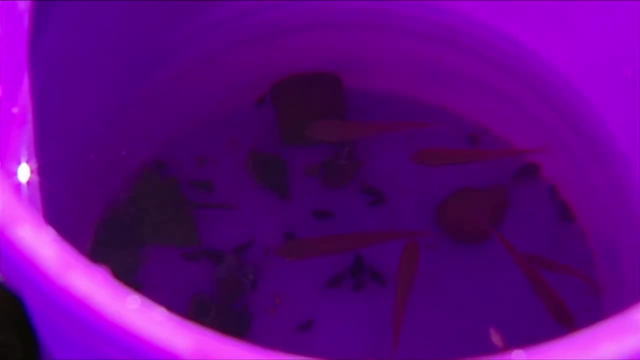 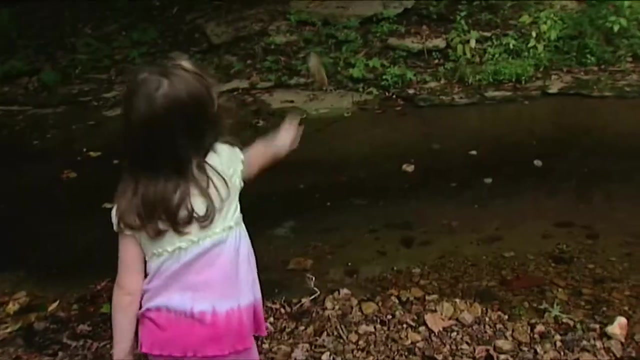 critters and little fish nets are great tools for a hands-on experience of life in a small stream, But be sure your kids understand the importance of setting captured critters free. Water's fun. dirt's fun. rocks are fun. trees and branches are fun- nature's fun.